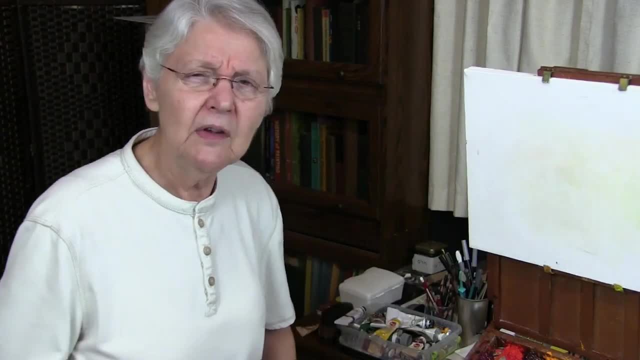 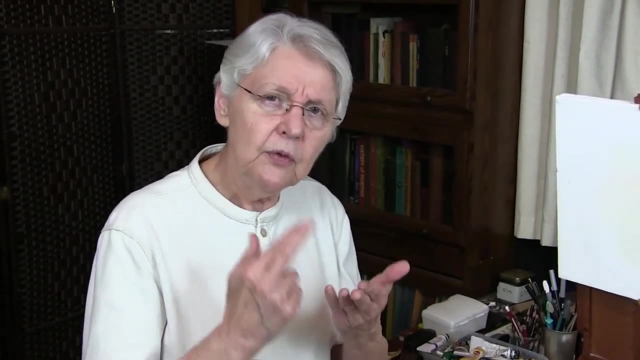 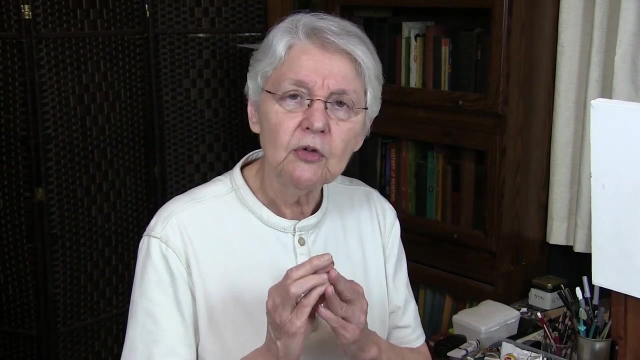 Light to dark, which can be very, very confusing. I have another way of thinking about value, and that is whether it's in shadow or not in shadow. And if you think about color, or if you approach color as to whether it's in shadow or not in shadow, then it enables you to. 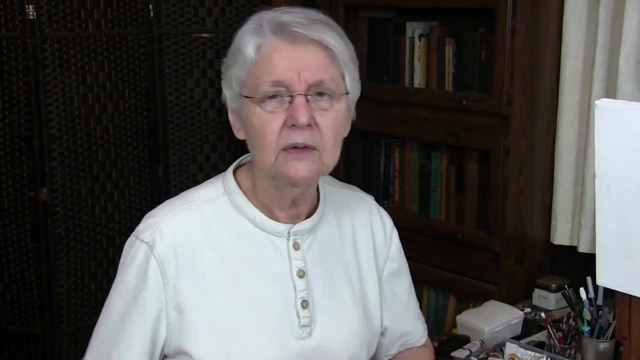 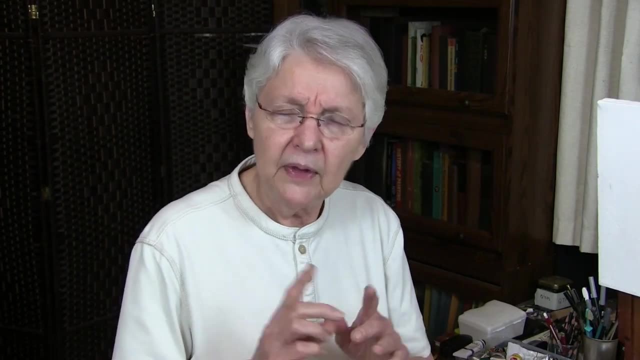 read the value of that color more clearly. It makes more sense. It makes a lot more sense to me to look at values in terms of shadows and not in shadows rather than in terms of numbers. So let's take a little bit of an analytical look at what I'm talking about. 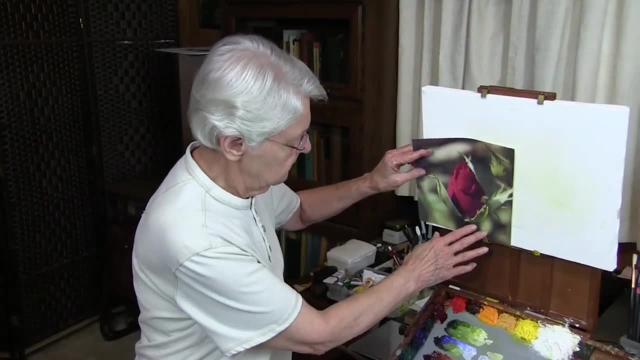 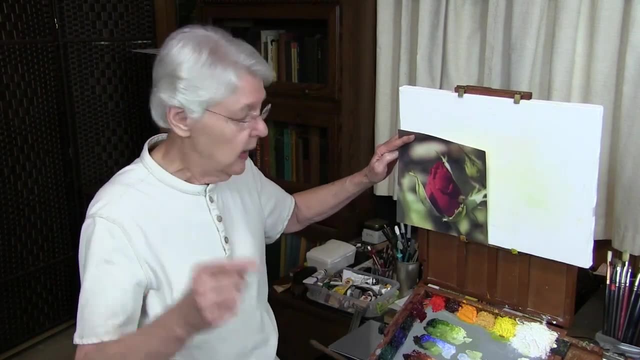 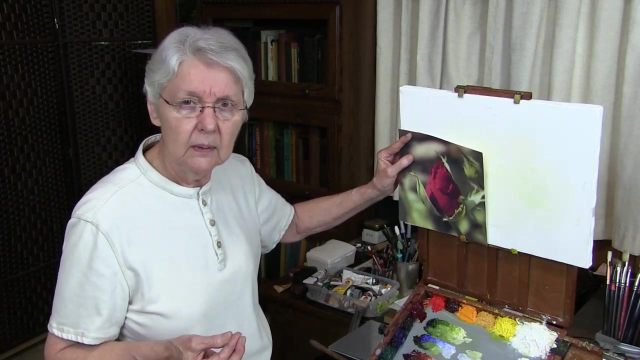 Now I have here a photograph of a rose. A rose, a red rose. We normally think of red being a lighter color. Let's say that a different way: A red rose in a green environment. Now, we usually think of a red as being a lighter color than green, But that's not true if the green is in light and the 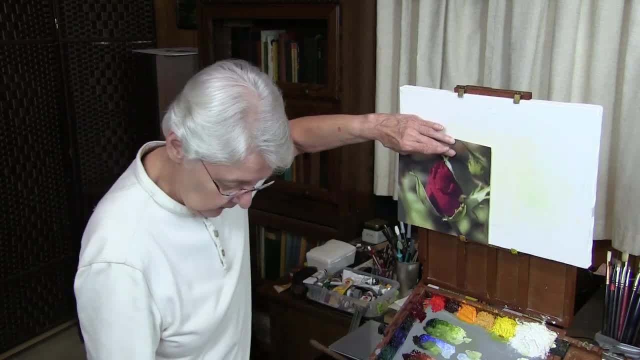 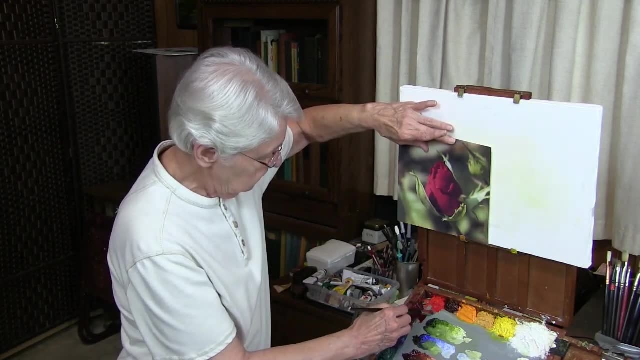 red is in shadow, And so you can see what I'm talking about. I'm talking about a rose in a green environment. Now what I'm talking about here, just with a little bit of an illustration. well, you see how light the red is on this side, And I'll give you just a little bit of an. 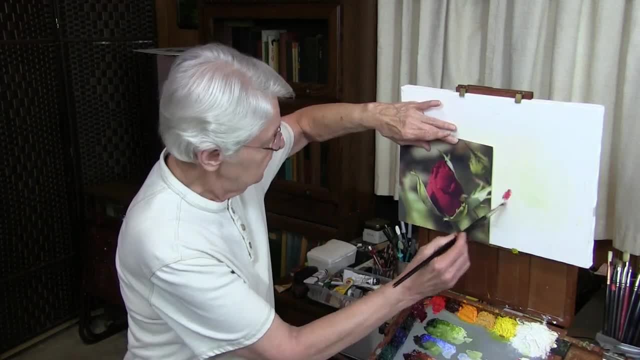 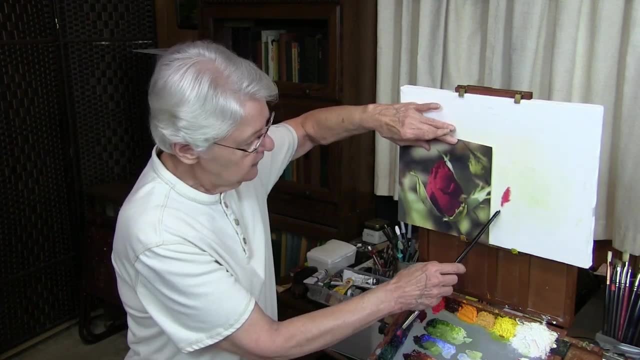 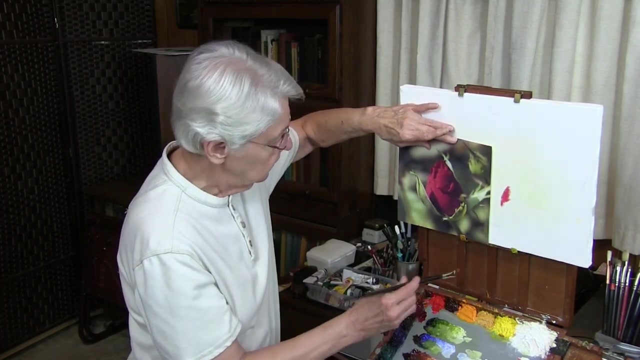 indication on the canvas here You see the light. The red here is about this light. Now when I put that light against this white canvas you see it seems a little bit darker than the canvas. But then when I put that red in shadow or I throw that red into the shadow color, if you look at 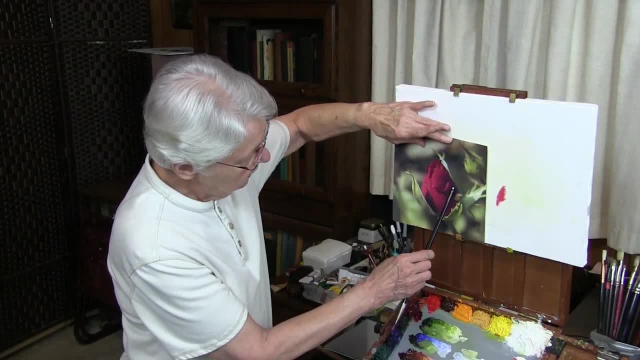 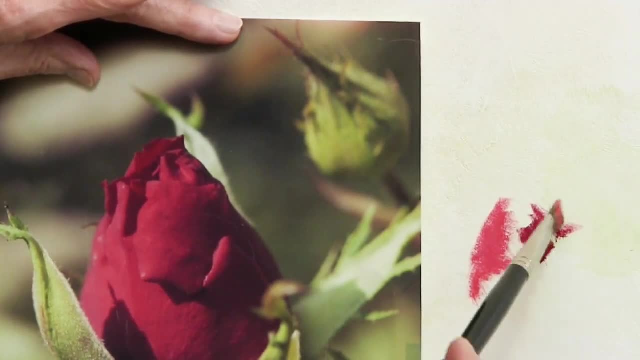 the shadow here. this cast shadow. you see that the red is a little bit darker than the canvas. Now you also look at the shadow on the opposite side of the red. You see that is quite dark, And so this is more like a shadow color of the red on the opposite side. In fact it is even darker than 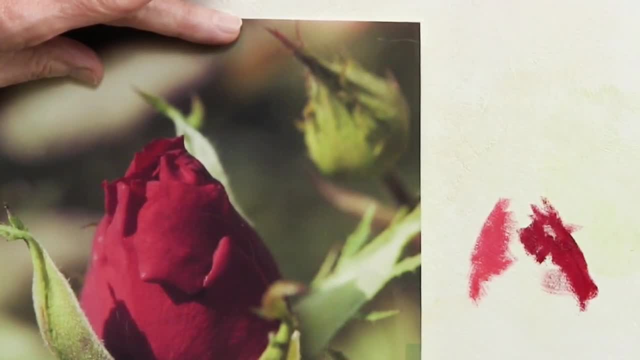 that, And so I'll just even darken that red a little bit more. I darken it by throwing a little green in it. Now, that is still red, Even though it's in the shadow side. it's still red, But it's. 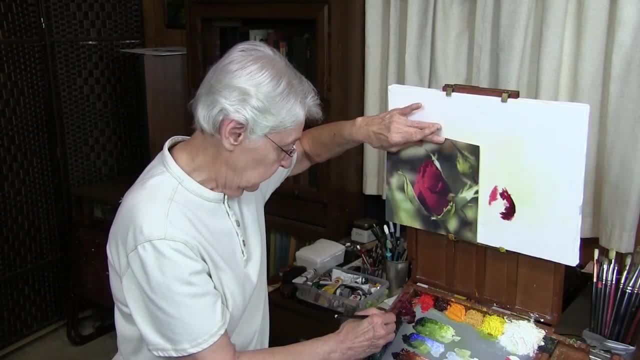 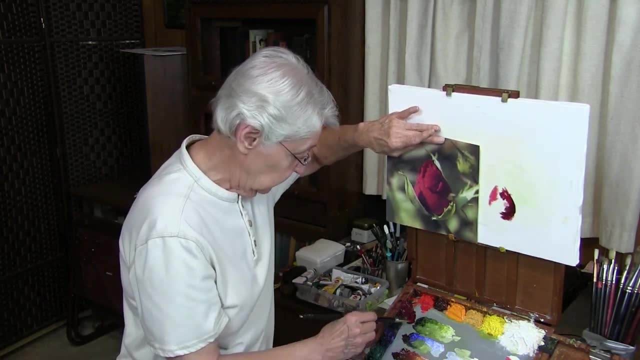 red in shadow. Now what we can do is that when things are in shadow, they can be in deep shadow. So let's look at what deep shadow might look like in red which we see there in that cast shadow. So deep shadow might look like. 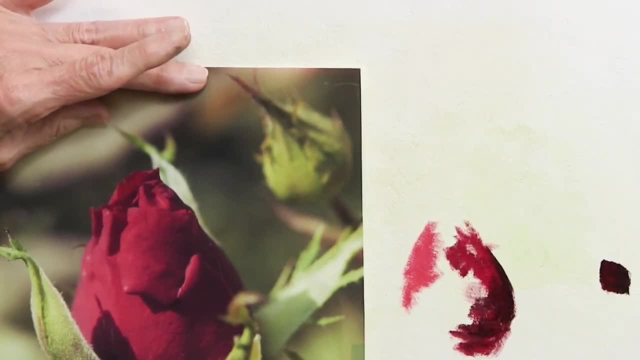 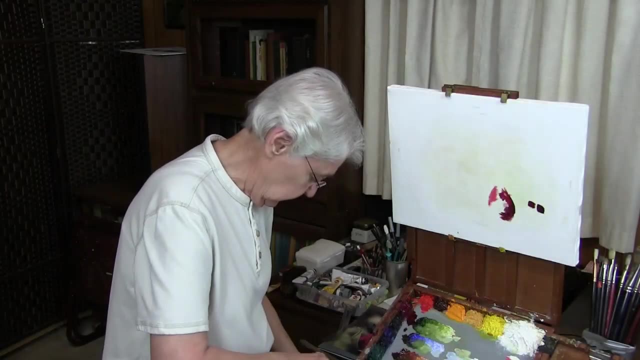 this Real, really dark. Then we might have more moderate shadow. that would look maybe a little bit like that- Not quite. Now I've got that a little bit dark. Let me just erase the brush and take that photograph down so I can have both hands to work with. 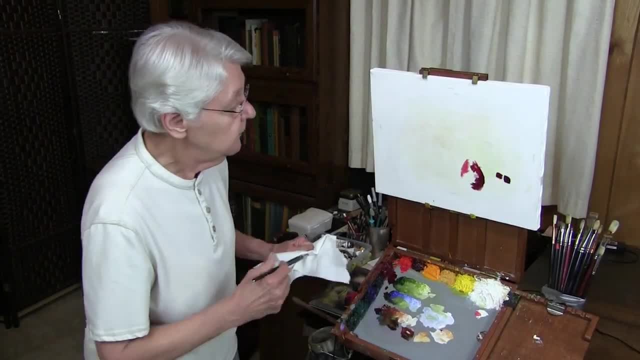 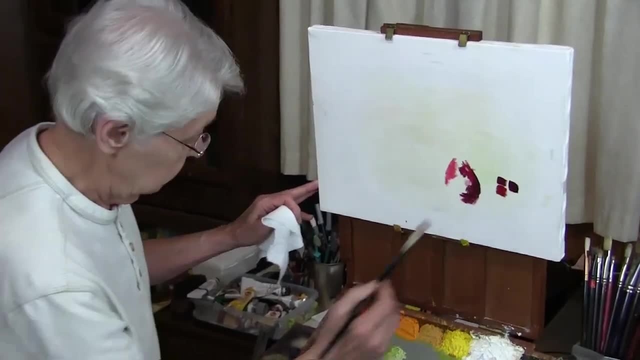 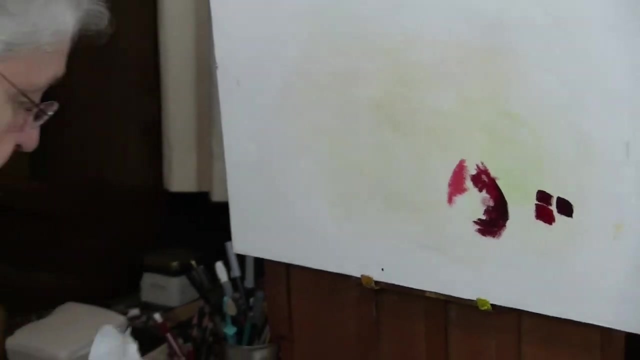 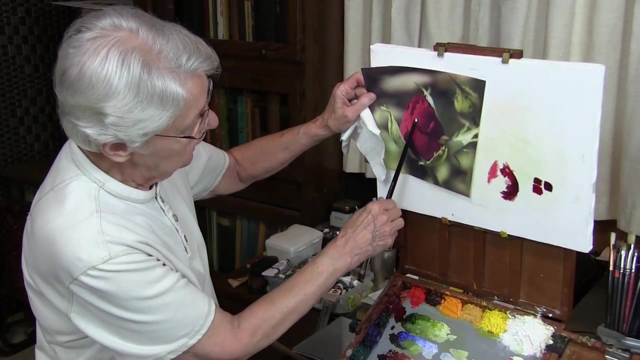 Okay, let's look at the moderate shadow. Moderate shadow might be something like that, Maybe a little bit darker, And then a shallow shadow. A shallow shadow- And if you can look back at the rose here, you see this falls into more shallow shadow where the rose turns away from the light source: Shallow shadow. 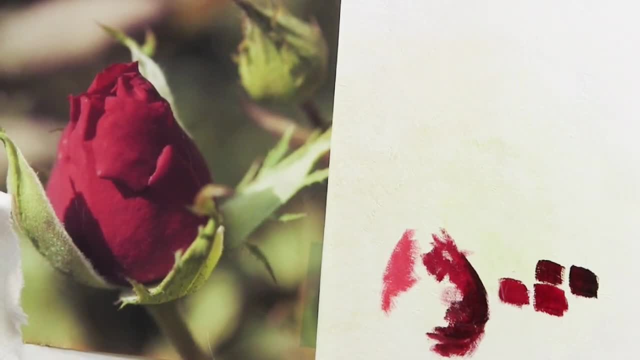 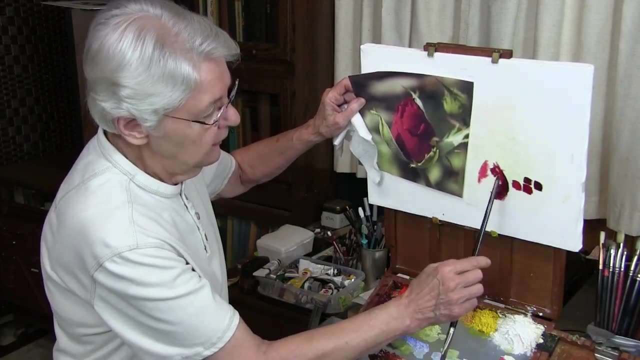 Then it would end up being a little bit lighter. Let's get that just a little bit lighter right there, So not a real good Shallow. then if you think of the values of shadow, the shadow side of red, the values as being 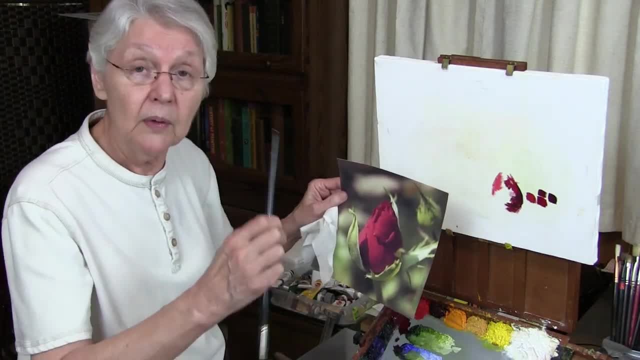 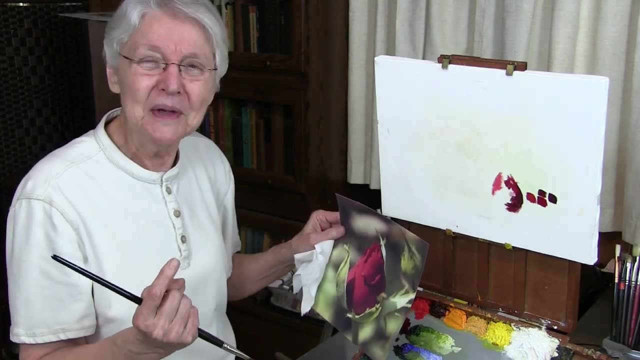 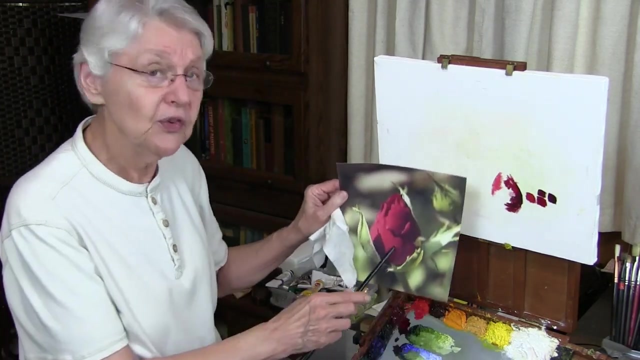 shallow, moderate and deep. that makes a lot more sense than if you say, okay, that's going to be values eight, nine and ten, If that's the value scale you're using, or if you said three, two and one if you were using the other value scale, which could be totally confusing. 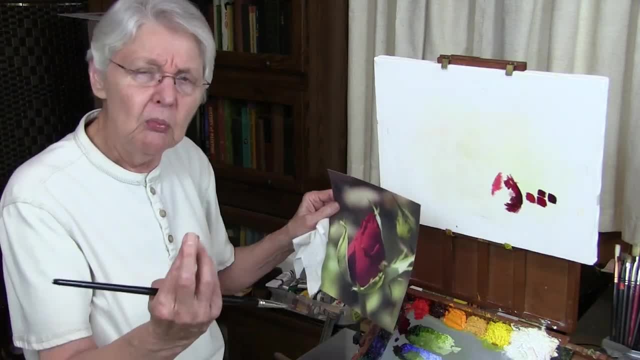 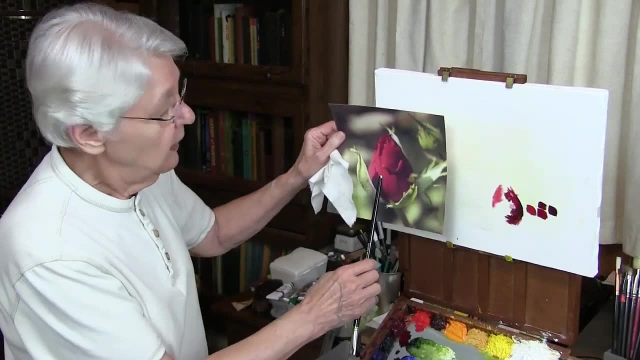 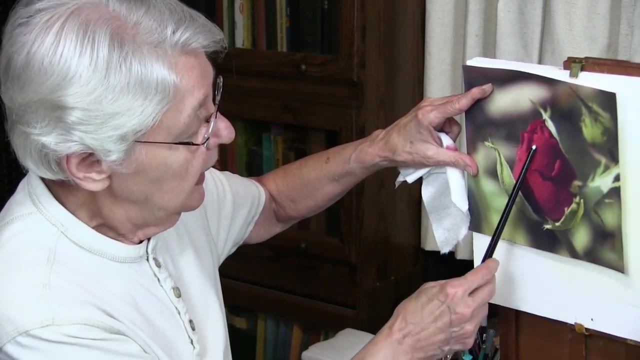 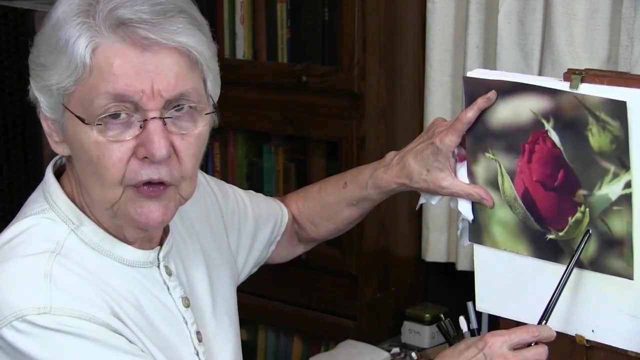 this won't be confusing. Now, as you're moving up the value scale with the color red, you'll reach that point where it's neither in shadow nor in light- Well, you might say the place where it crosses from shadow into light on something that's a round form like the rose. we call that the. 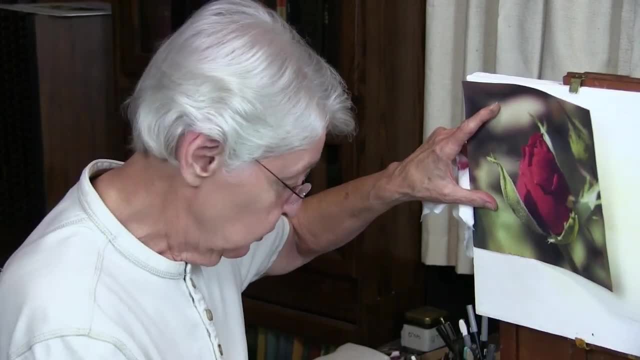 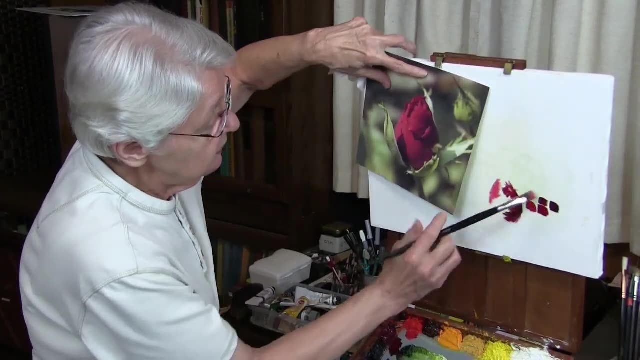 terminator line, And that is the place where we read it as red. that's the place where it's called the value of the color that it is, And so in this case, if we just throw this red here, this is a natural red straight out. 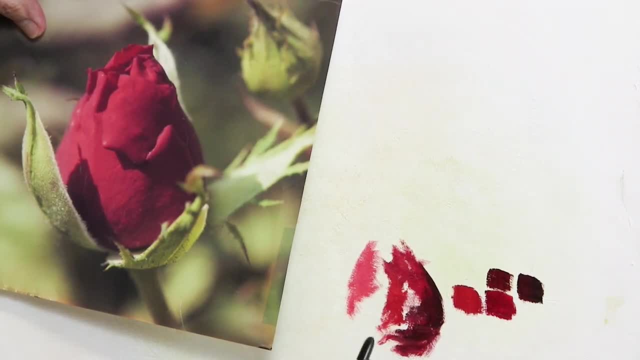 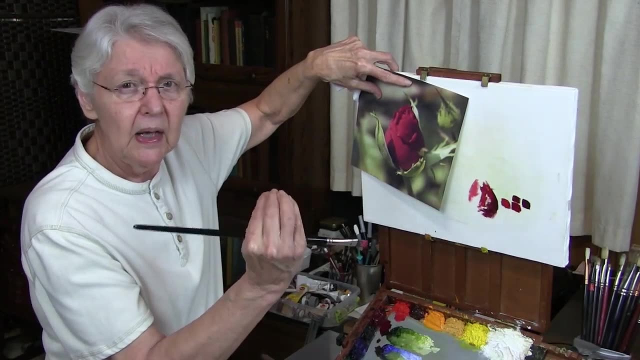 of the tube, like right there, that then indicates the, the color of the, the of the rose itself. Then, as it moves towards light, it begins to get lighter. And so, as it moves towards light, it starts to get lighter, And so as it. 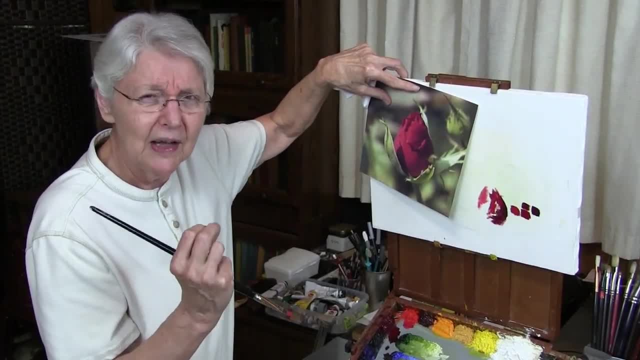 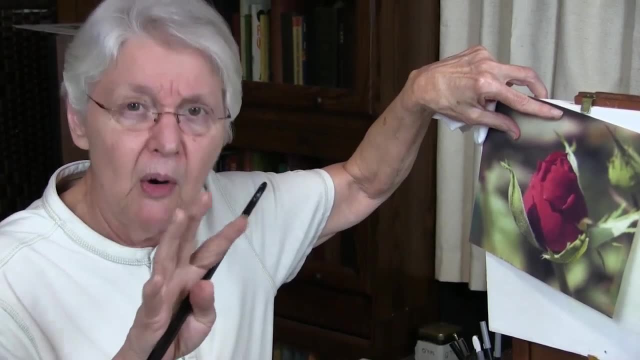 and where it's being hit directly by light, it's going to be very, very, very light. So you've got center light, where it's very, very light and light red, and then you've got what we call half tones or mid-tones. 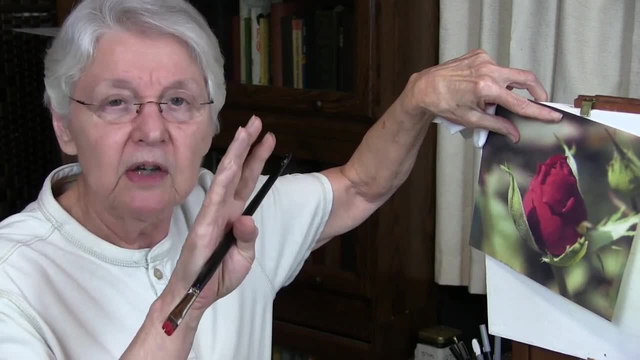 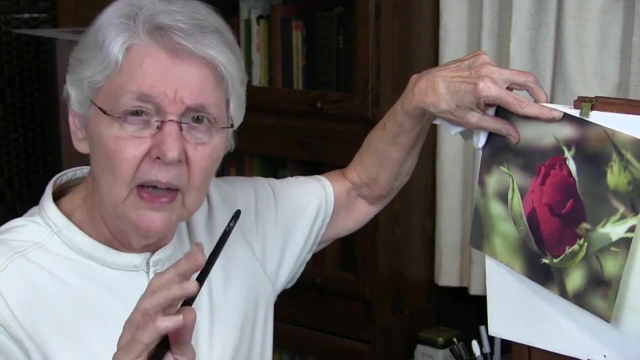 that would start with, right where the center light is. It gets a red, would get a little bit lighter or a little darker- less light, I should say- And then, as it moves towards that terminator, it begins to pick up a little bit more color, more value. 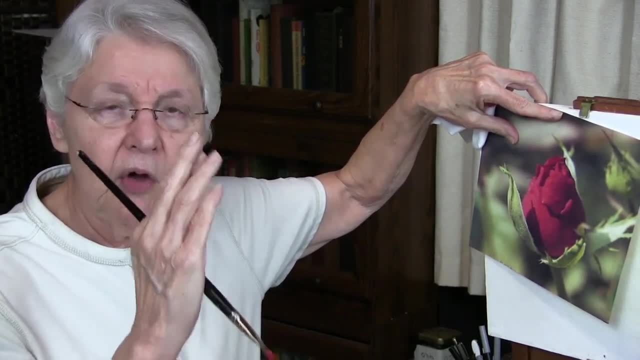 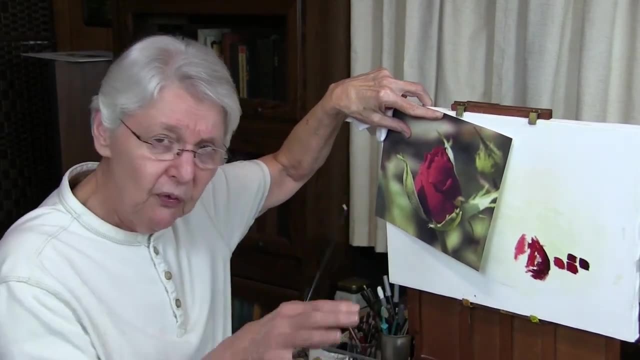 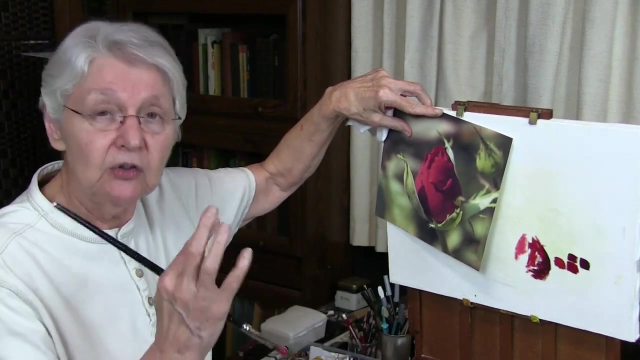 So it would be like center light: half tone one, half tone two, or half tone three. when it reaches this point of just before it turns into shadow. So in that case we might say red is light. Red hit by light is going to be lighter than red that's in shadow. 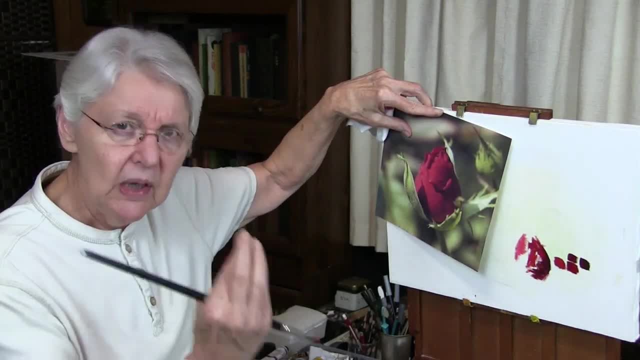 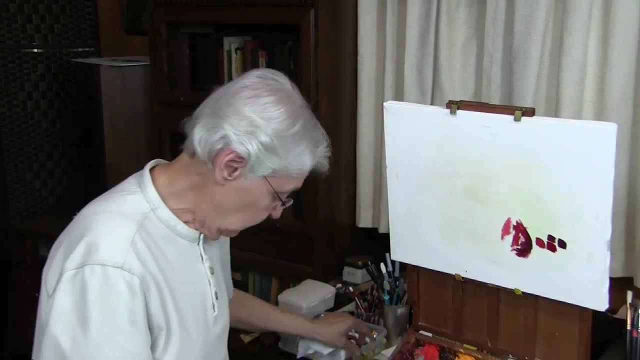 So you see, it's all relative and when you read it that way, whether it is in light or whether it's in shadow, it makes a lot more sense. One more thing, One more little point I want to make here. Let me rinse the brush out. 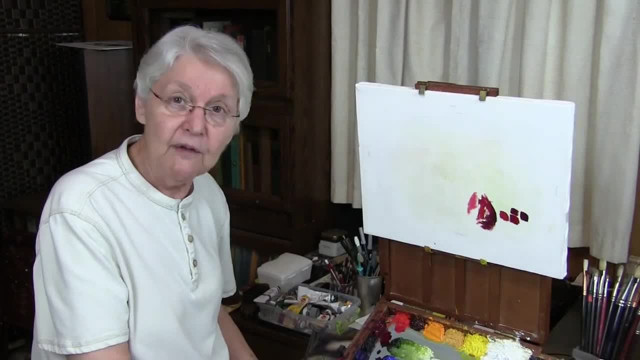 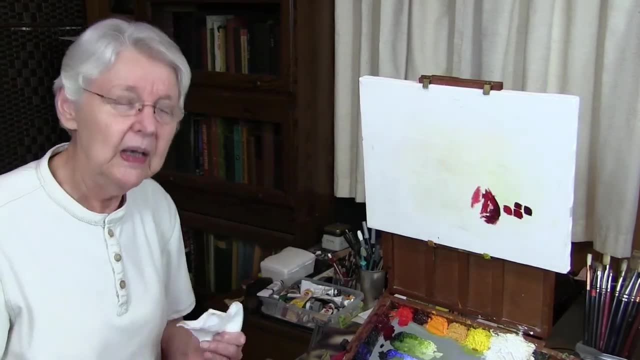 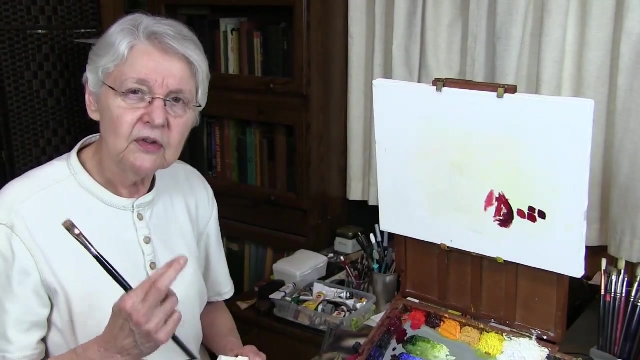 And that is the original point I brought up of red versus green. Now we usually we would think if I said to you which is darker, red or green, You might say green is darker. Well, that's not a really good question, because red versus green. 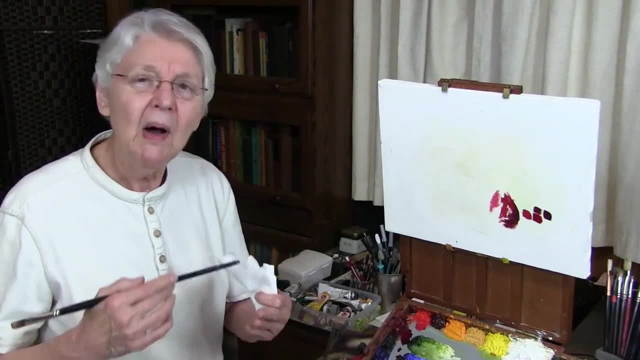 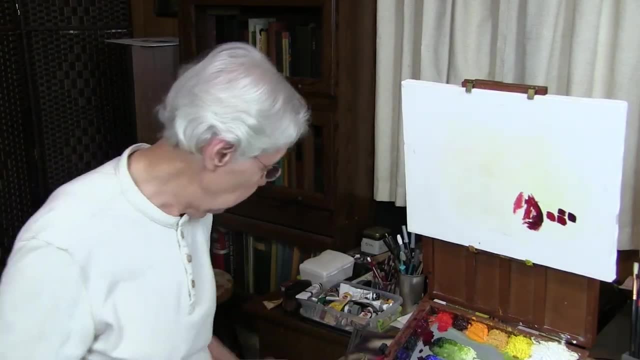 no matter what color will be determined by how much light is shining on the color or how much It's in shadow, to what degree it's in shadow, And so you can see right here. you see right here where this green is being hit very 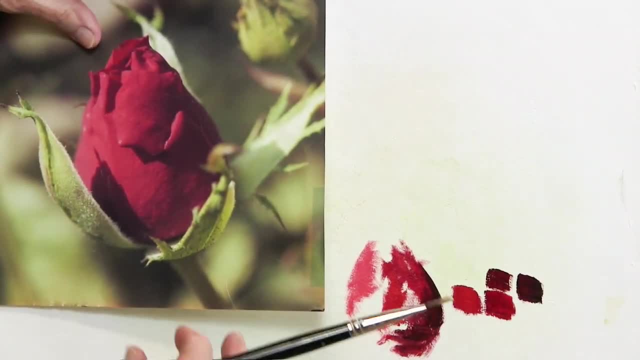 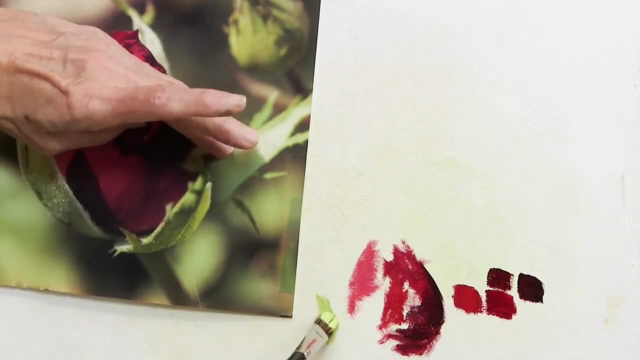 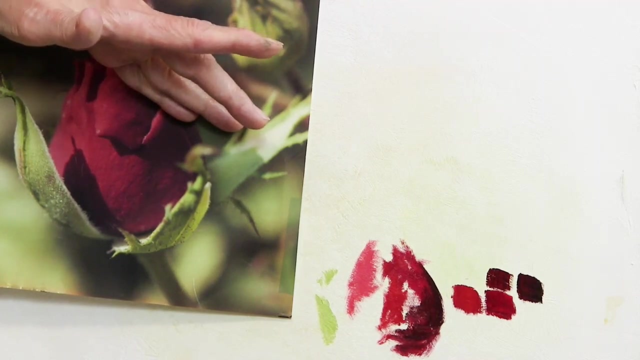 very strongly by light. it's light green. It's more like more like this: this color of green or this value of green. you should say this value of green right here, where it's being hit very, very strongly by light. as that moves into shadow it will become darker. more like this: 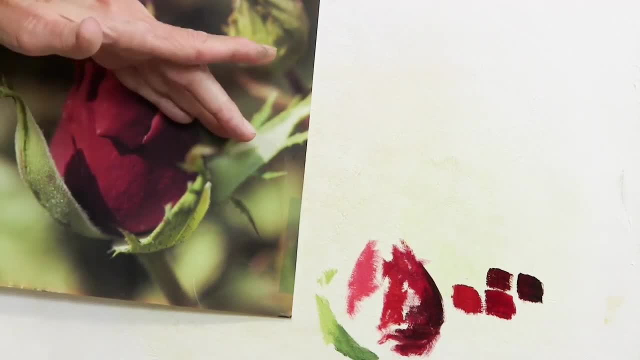 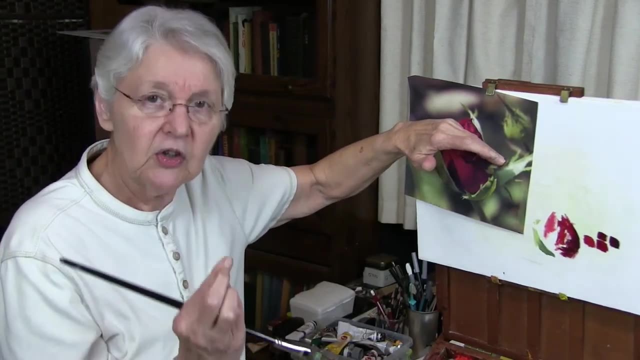 You see, This is darker green because it's moving more towards in shadow. This is the lighter green because it's moving more towards light. Now we're talking just about value here. We're not talking about reflected light and all those kinds of things, just the value of color.